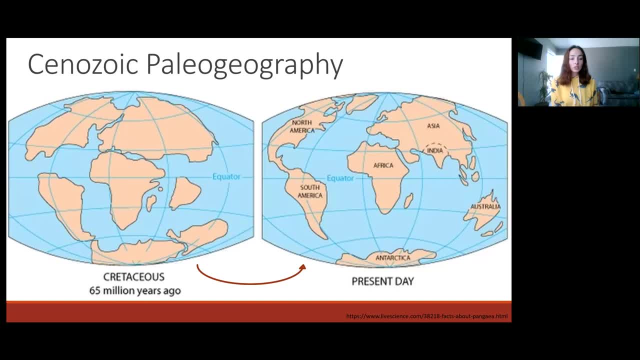 it's not in the Mesozoic. So we're going to start with the Cenozoic and we're going to. India was still moving up to collide with Asia and hadn't done so yet, and Australia and Antarctica were still kind of locked together and hadn't really separated much yet. So these were the. 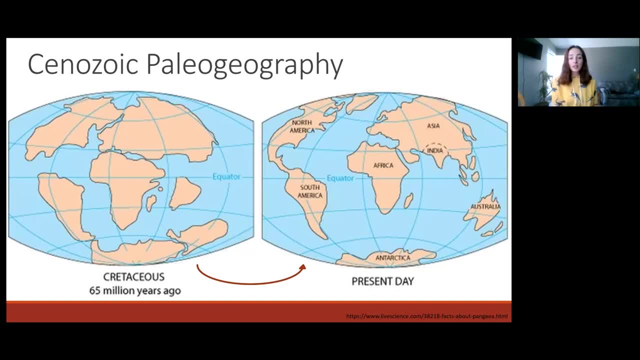 main two movements, but basically the configuration of continents finalized itself during the Cenozoic. So now let's look at what's happening at the surface throughout the Cenozoic and how it led to our current tectonic situation throughout the globe, as well as the current mountain belts that 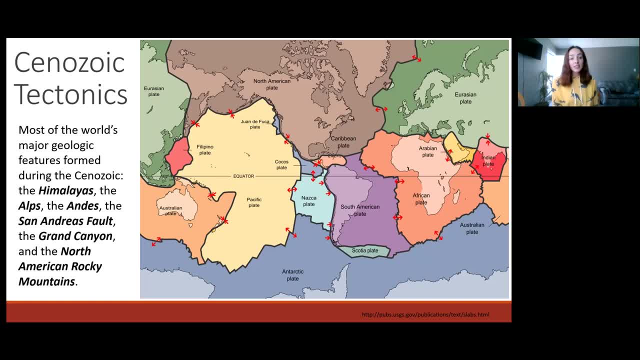 we have at our surface today. So here's the current configuration of a lithospheric plates on Earth today and where they are colliding with each other. During the Cenozoic, most of the world's geologic features were formed or are still being formed, including the Himalayas. 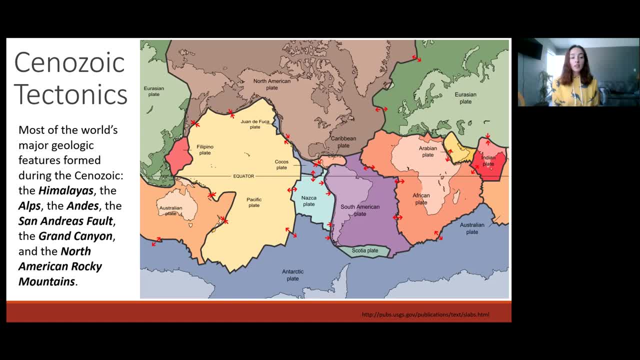 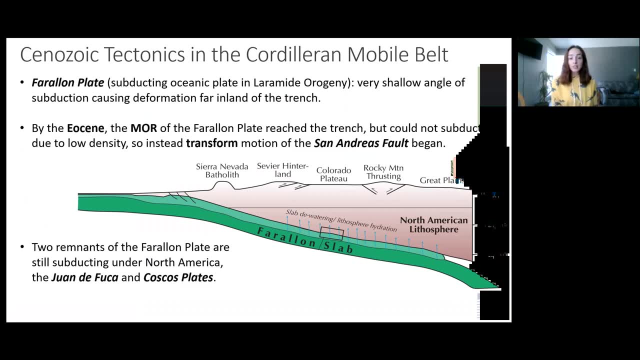 the Alps, the Andes, the San Andreas Fault, the Grand Canyon and the North American Rocky Mountains. To start with, we're going to talk about the tectonics that were occurring at the Cordilleran Mobile Belt throughout the Cenozoic and what's occurring now at that mobile belt. 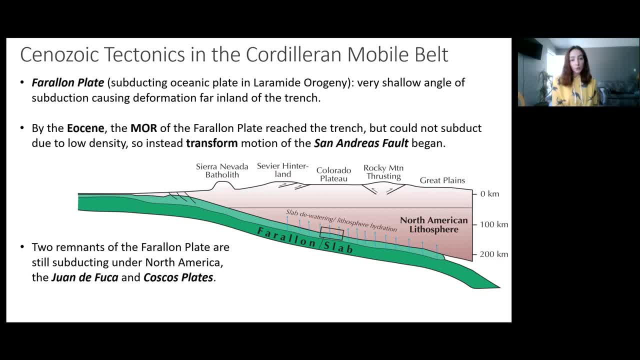 We talked about how the Cordilleran Mobile Belt is at the western margin of the US. In the last video over the Mesozoic, we talked about how the Nevadan and severe orogenies occurred in the Mesozoic and we talked about how the Laramide Orogeny began. 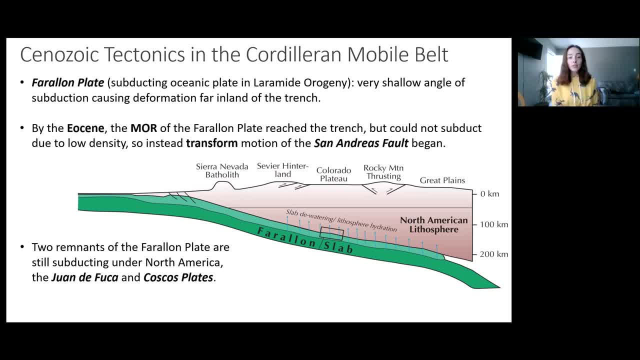 in the Mesozoic, but then continued until the Eocene. The Laramide Orogeny was the last major orogenic event contributing to the development of the Cordilleran Mobile Belt before a change in stress occurred. Basically, the Laramide Orogeny was the subduction of the 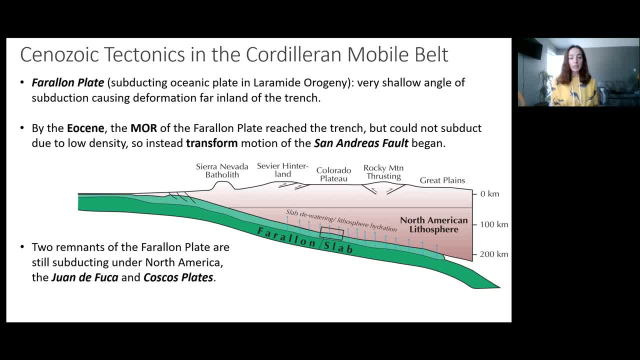 Farallon Plate, an oceanic slab that subducted under North America at a very shallow angle, causing deformation further inland of the trench, And then by the Eocene. the subduction got to the point where the mid-ocean ridge of the Farallon Plate had reached the trench. However, that was 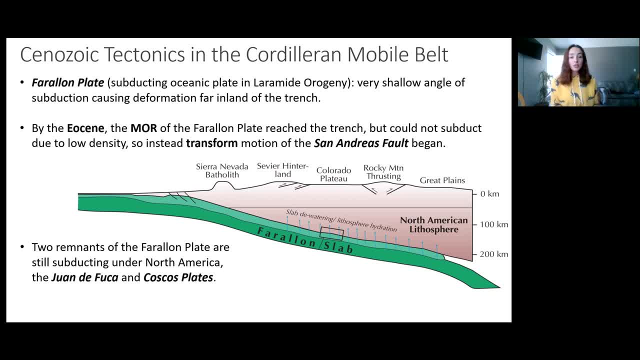 the point at which subduction ceased, And this is because the mid-ocean ridge wasn't dense enough to subduct and therefore the stress changed from compressional to shear, And that was because transform motion began causing the San Andreas Fault instead of continuing compressional subduction. 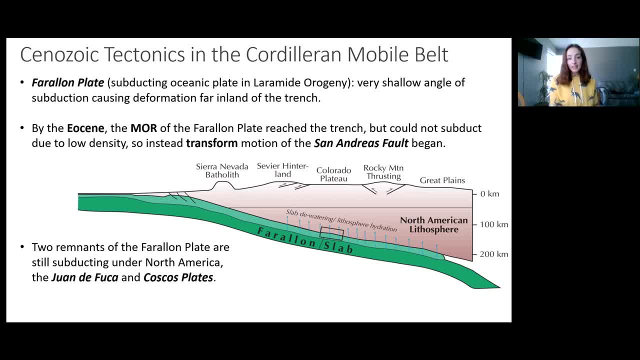 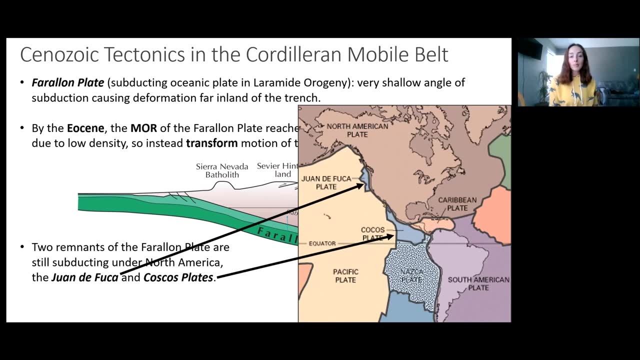 Currently today, the remnants of the Farallon Plate that hadn't subducted, yet called the Juan de Fuca Plate and the Cuscus Plate, are still subducting under North America, as seen in this map. However, the shift in stress regime in the Eocene did cause a lot more that I want to talk about. 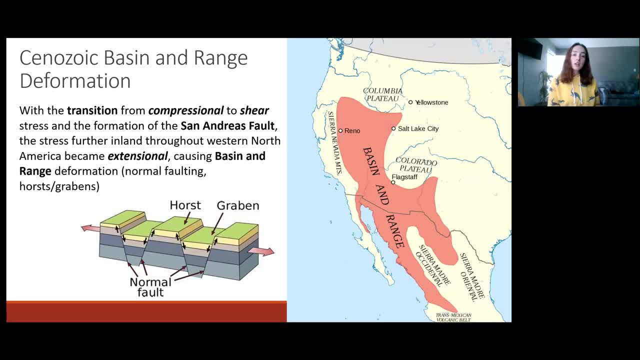 before we move on to more recent events. So let's talk about the basin and range deformation During the Eocene, when the transition of compressional to shear stress began, the stress further inland out western North America became extensional And this caused basin and range deformation. 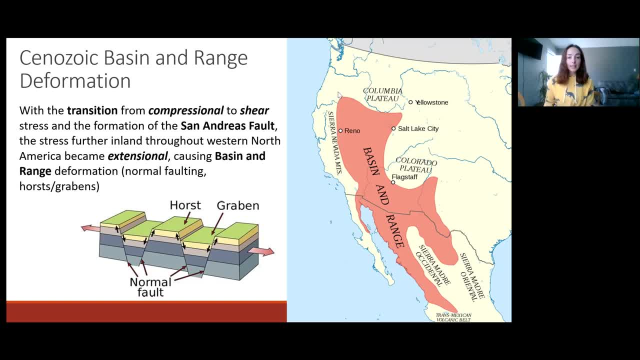 Basically all the compressional deformation that had occurred further inland due to the Farallon Plate subduction at a low angle that had just switched from compressional to extensional, causing all the compressional fold and thrust deformation to become basin and range deformation where extensional normal faulting and Horsts and Grobbins formed. 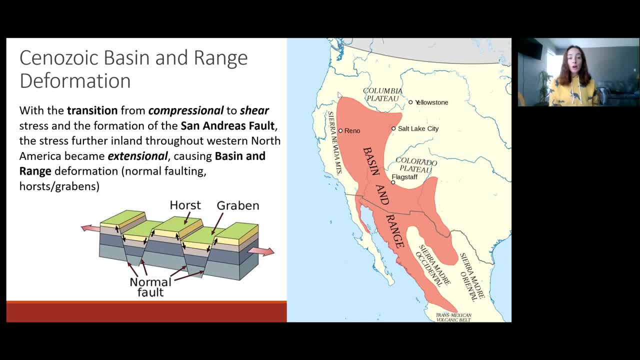 Horsts and Grobbins are basically in this lower picture. we can see that the Grobbins are dropped down blocks due to normal faults on either side of a Grobbin, and Horsts are the blocks that don't drop down or are even uplifted in some cases. So, along with the extension during this time, 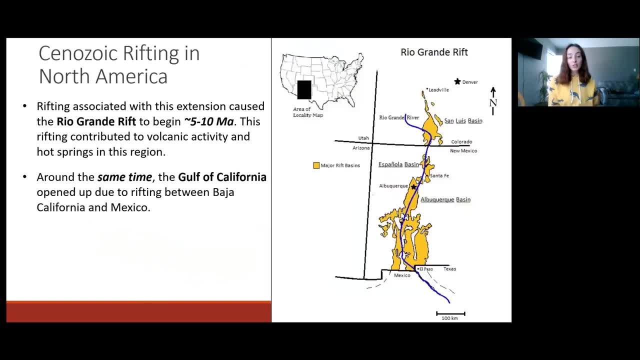 and in this area, we also had rifting occur in North America. However, these two specific instances I'll be talking about were much later. For example, the Rio Grande Rift began around five to ten million years ago, and this rifting is shown in the right picture, where we have the yellow blob. 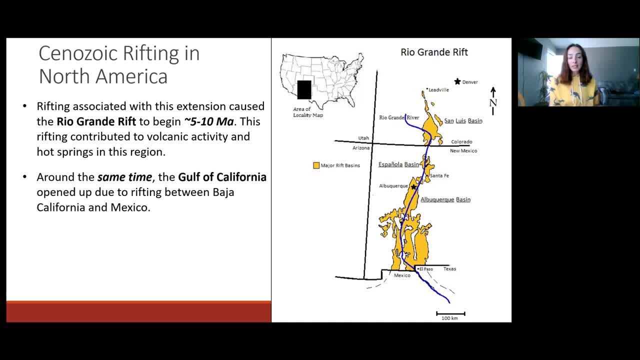 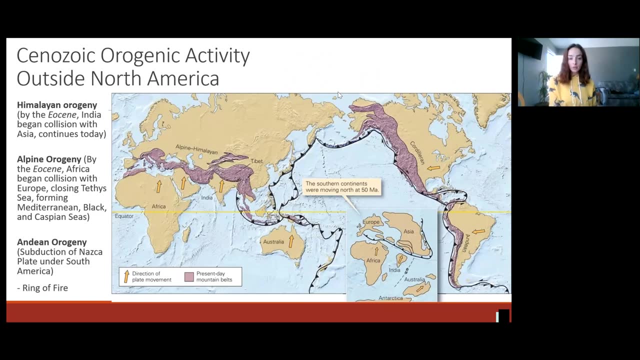 and then we have the Rio Grande River in the rift valley. We also had, around the same time as this rift, the rifting between Baja California and Mexico, causing the Gulf of California to open up, which is shown here. So, moving on to orogenic activity outside of North America, this is a map. 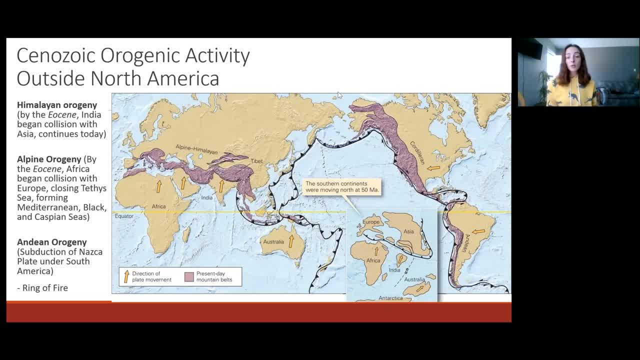 showing in purple the Alpine and Himalayan Mobile Belts, the Cordilleran Mobile Belt and the Andean Mobile Belt. We just talked about the Cordilleran Mobile Belt and the deformation it caused in North America during the Cenozoic. 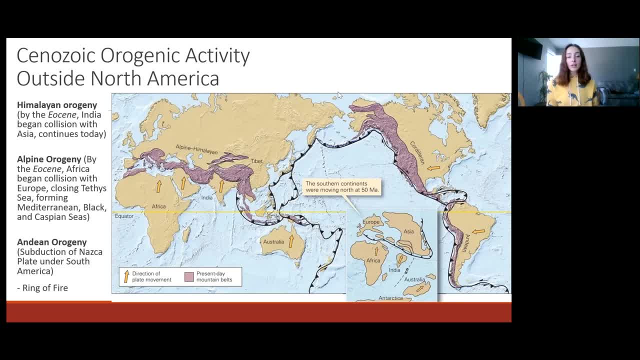 However, let's now turn our attention to outside of North America, for example, the Himalayan, the Alpine and the Andean orogenies. The Himalayan orogeny began around the Eocene when India collided with Asia, and is continued today, as India continues to push toward Asia. The Alpine 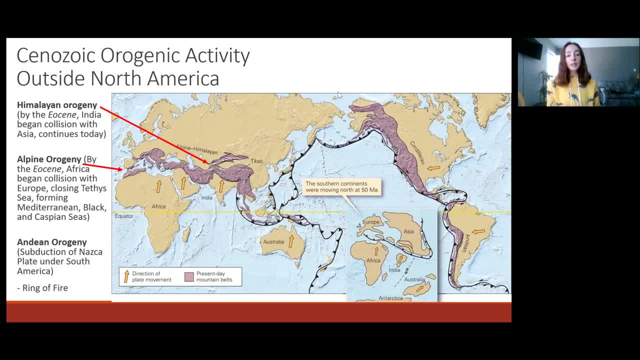 orogeny also began by the Eocene, as Africa began colliding with Europe, closing the Tethys Sea and forming the Mediterranean, Black and Caspian Seas. If you don't remember what the Tethys Sea was, remember when we went over the continental configurations during the Mesozoic, right after. 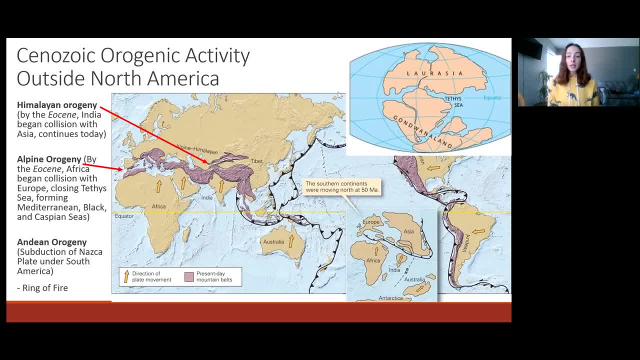 Pangea formed during the latest Paleozoic. we had Pangea break up back into Laurasia and Gondwana land, forming the Tethys Sea in between these two continental masses. and this Tethys Sea remained in between Europe and Africa until Africa closed that gap and the remnants of the Tethys Sea are. 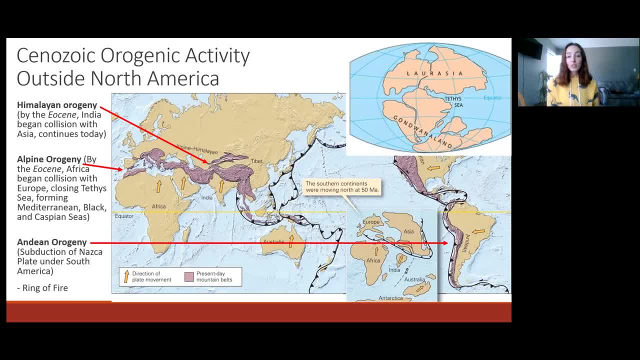 the Mediterranean, Black and Caspian Seas. Now the Andean orogeny is caused by the seduction of the Nazca Plate and the Caspian Sea, and the Caspian Sea is caused by the seduction of the. 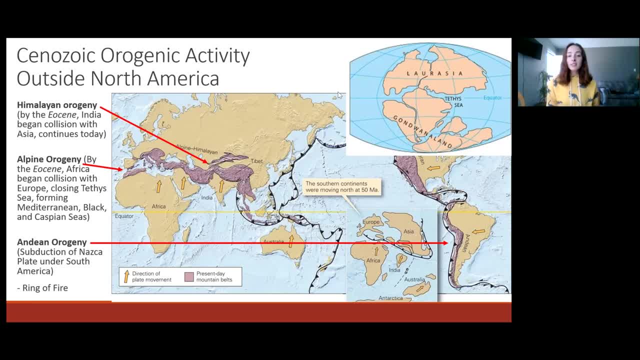 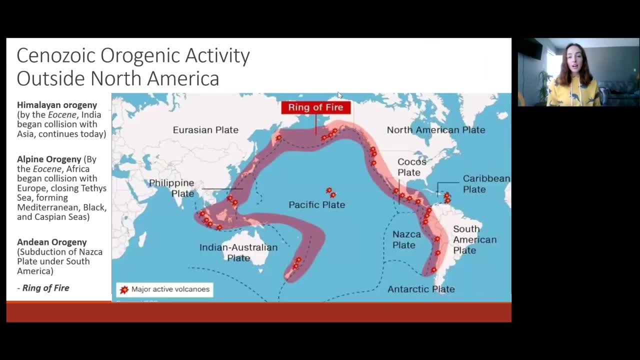 Andean orogeny under South America and continues today as well. And another thing that all of the ocean-continent subduction zones are famous for on Earth today is something called the Ring of Fire. The Ring of Fire is defined by strong earthquakes and intense volcanic activity that occurs along 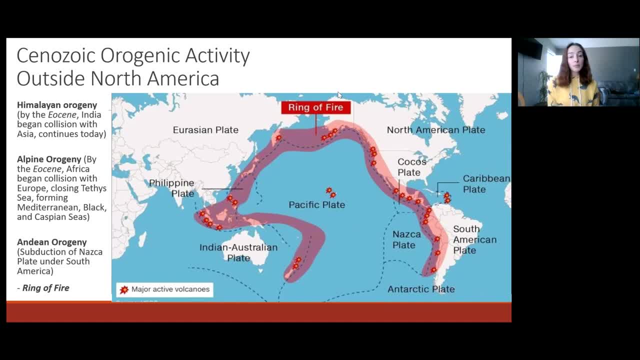 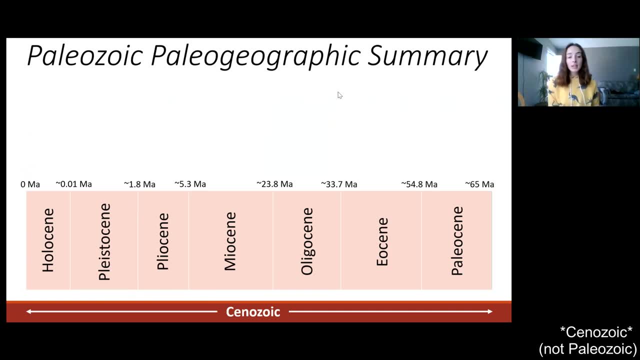 ocean-continent subduction zones along the margins of the Pacific Ocean. Now, to just give a brief summary of the geologic events that we just discussed, let's put them all along the timeline of the Cenozoic Era. The Cenozoic Era is a geologic event that takes place in the Pacific Ocean. 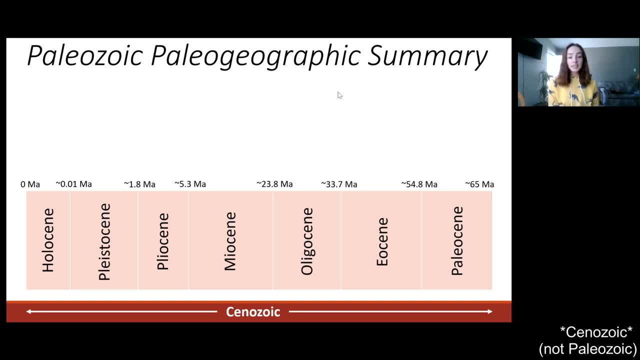 Now to just give a brief summary of the geologic events that we just discussed. let's put them all along the timeline of the Cenozoic Era. The Cenozoic Era has epochs: Paleocene, Eocene, Oligocene, Miocene, Pliocene, Pleistocene and Holocene. 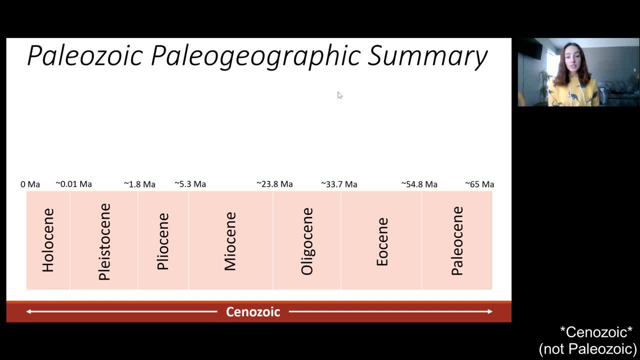 and these epochs go from 65 million years ago, at the end of the Mesozoic, to now at the end of the Holocene, at 0 million years ago. as we are in the Holocene currently, So going from right to left, we have the Andean orogeny beginning in the earliest Paleocene. 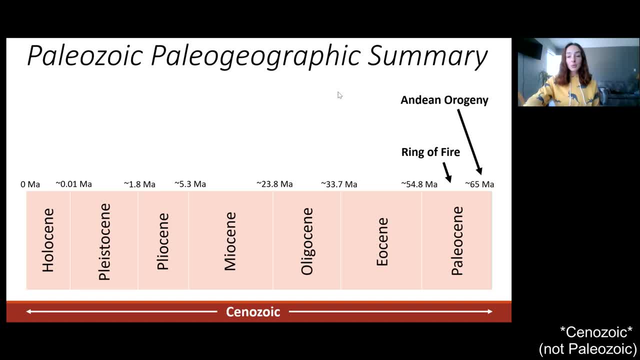 the Ring of Fire also beginning to form around this time as well, due to subduction zones such as the Andean, the Himalayan orogeny beginning in the Eocene, the Laramide orogeny ending in the Eocene. remember it started in the late Mesozoic. 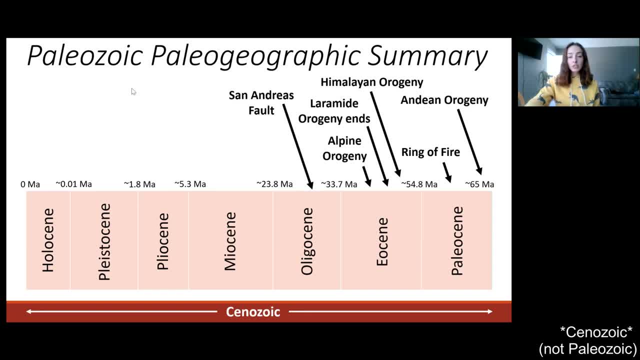 the Alpine orogeny beginning also in the Eocene. the San Andreas Fault forming due to the end of the Laramide subduction and beginning of shear stress. the beginning of the Basin and Range extension. the beginning of Central America subduction. the beginning of the Rio Grande Rift Zone. 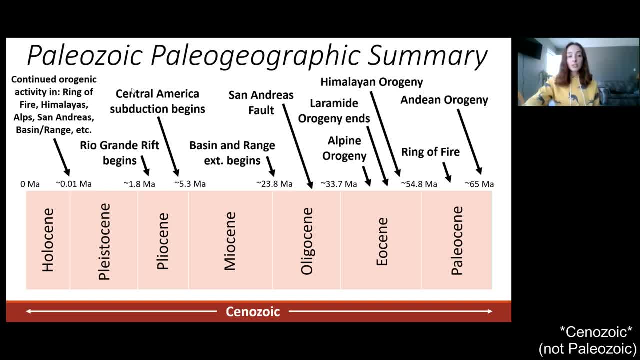 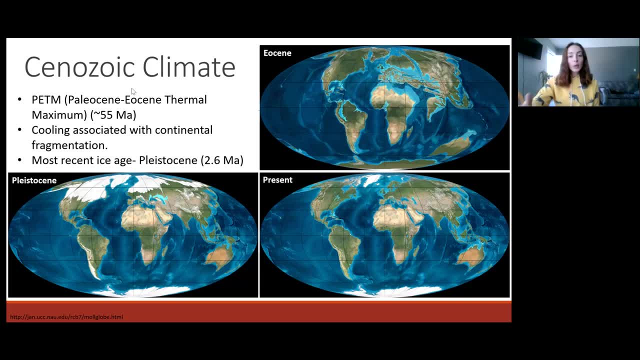 and the Ring of Fire, the Himalayas, the Alps, the San Andreas and the Basin and Range continue in their orogenic activity today. So now, before we get to the biological events that occurred in the Cenozoic, let's just talk about the climate a little bit. 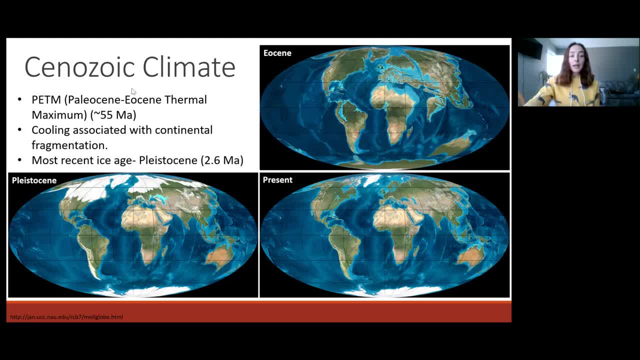 The climate in the Cenozoic began pretty hot and the Paleocene-Eocene boundary is marked by a thermal maximum, meaning a really hot period around 55 million years ago. However, the rest of the Cenozoic era up until today has been marked by pretty intense cooling associated with continental fragmentation. 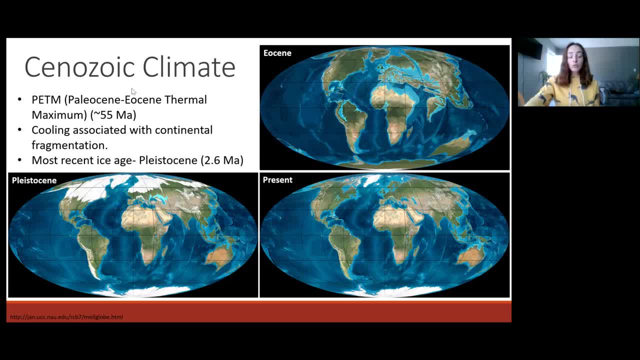 and then we had our most recent ice age, happening around 2.6 million years ago in the Pleistocene, and ever since then things have been warming up again, And now, of course, we're adding on to that. But besides that, these are the transitions of the Cenozoic in terms of climate. 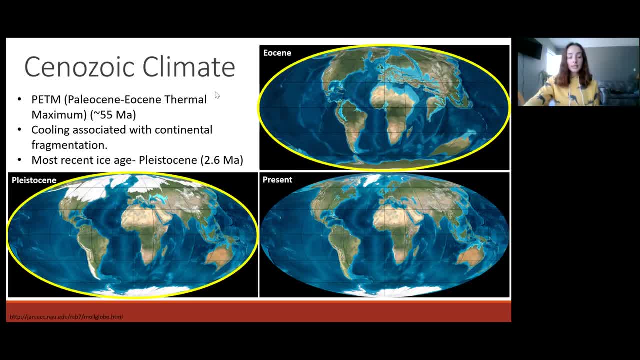 We have the Eocene warm period with high sea level. we had the Pleistocene, way later with the ice age, and now we have the present with ice caps but more temperate temperatures and sea level throughout most of the globe. Now moving to Cenozoic life. 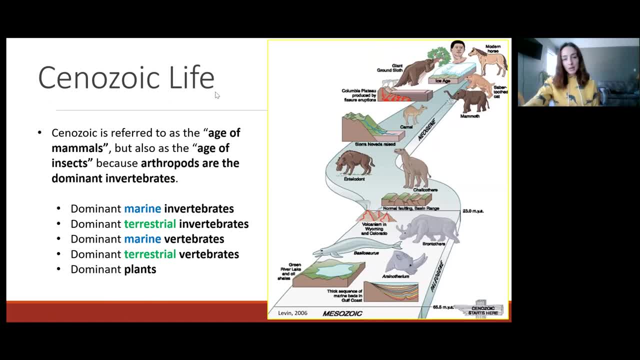 the Cenozoic is referred to, in terms of vertebrates, as the age of mammals, and can also be referred to in terms of invertebrates as the age of insects. These are the two main dominant types of organisms for vertebrates and invertebrates respectively. And so now let's talk about the events that occurred evolutionarily and 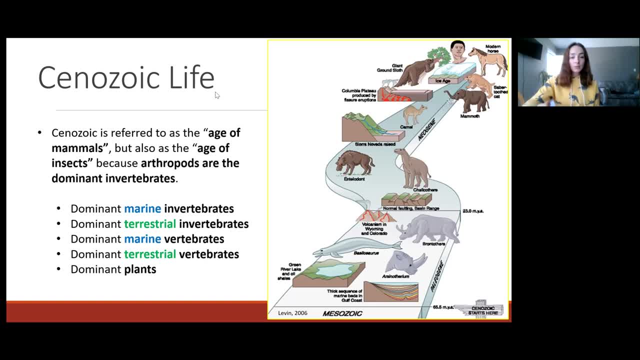 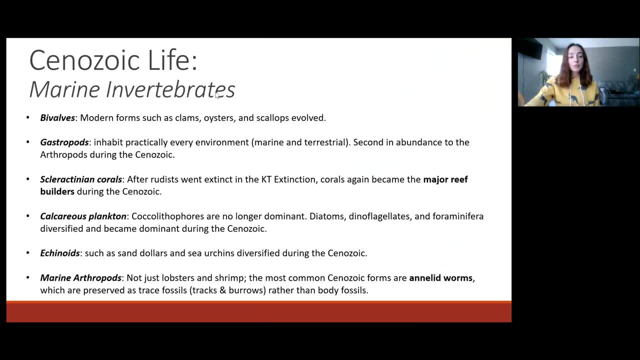 biologically for the marine invertebrates, the terrestrial invertebrates, the marine vertebrates, the terrestrial vertebrates and then the plants. So, starting with the marine invertebrates, we had the modern forms of bivalves such as clams, oysters and scallops evolve. We had gastropods. 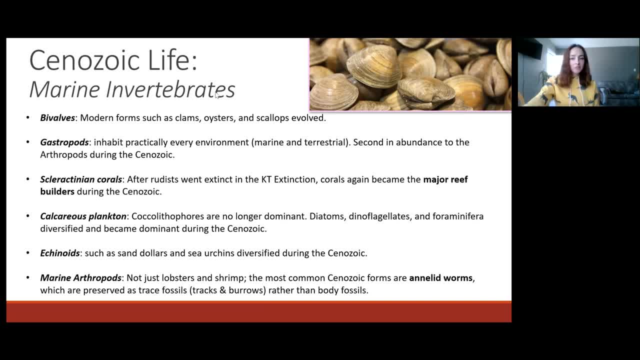 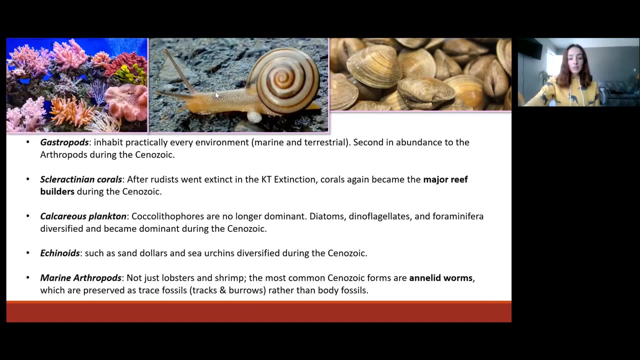 expand to inhabit practically every single marine and terrestrial environment, And gastropods also represent the second most abundant invertebrate during the entire Cenozoic, second right behind arthropods. And then we had sclerotinian corals. After the rudest wind extinct sclerotinian corals. 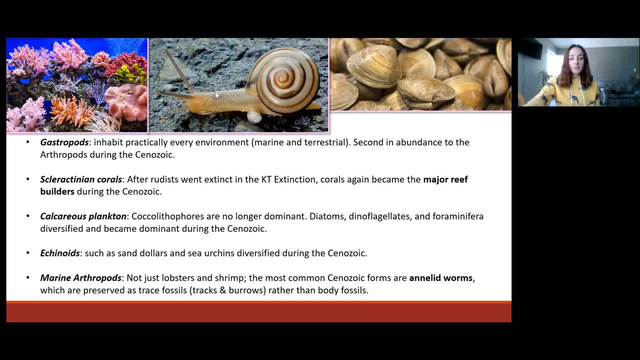 were able to become the major reef builders again and ever since then have been dominating reef building and reef communities in marine environments. And then we also have calcareous microplankton. We talked about calcareous microplankton in the past, but we also have calcareous microplankton in the 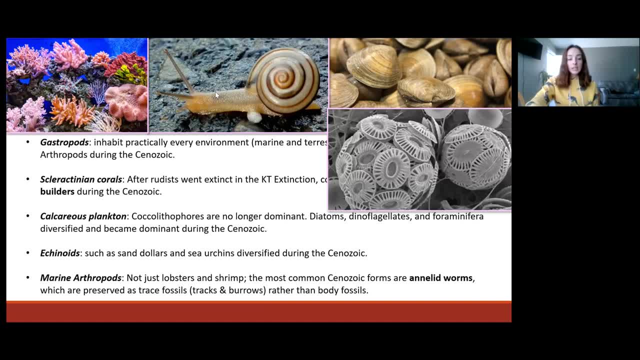 Mesozoic being dominant in the Cretaceous and causing the Cretaceous to be named after the rock they form, which is chalk, and in Latin that is creta. However, in the Cenozoic coccolithophores, 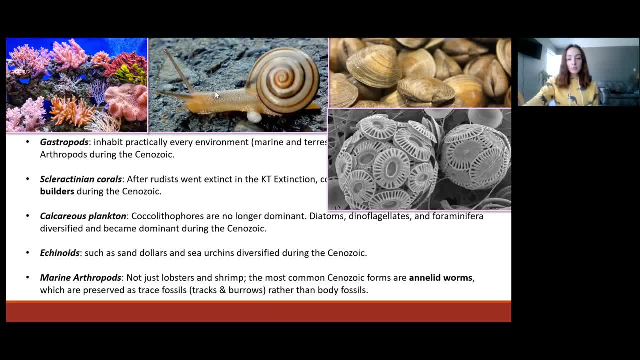 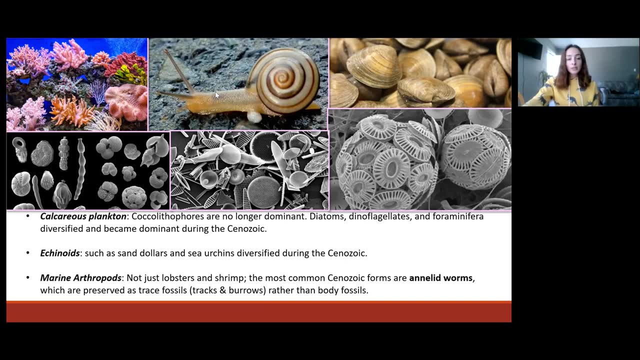 were no longer dominant. Actually, the dominant forms of calcareous plankton were diatoms, dinoflagellants and foraminifera. These are just other groups of microorganisms that grow their skeletons or tests or shells, whatever you want to call it, with calcium carbonate. Then we also 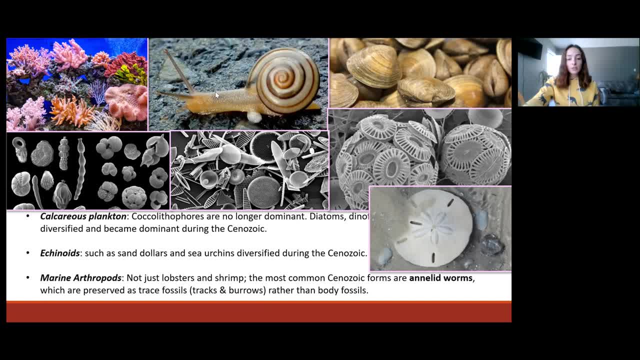 have echinoids such as sand dollars and sea urchins diversify in Cenozoic, And then we had marine arthropods And arthropods in the ocean. you might think about lobsters and shrimp, but they were much more than this. The most common Cenozoic forms are annelid worms, which are not preserved. 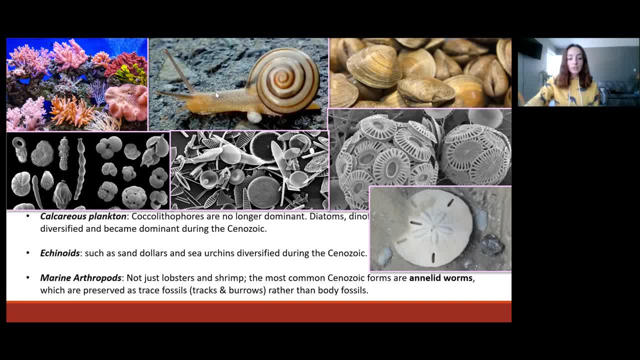 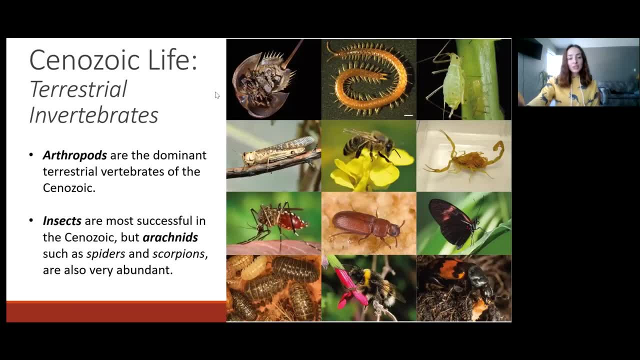 as body fossils, but are preserved most often as trace fossils, forming tracks and burrows in the sediment. So now let's move on to terrestrial invertebrates, which we already mentioned at the beginning of the Cenozoic life cycle, And then we have the arthropods in the ocean, which are 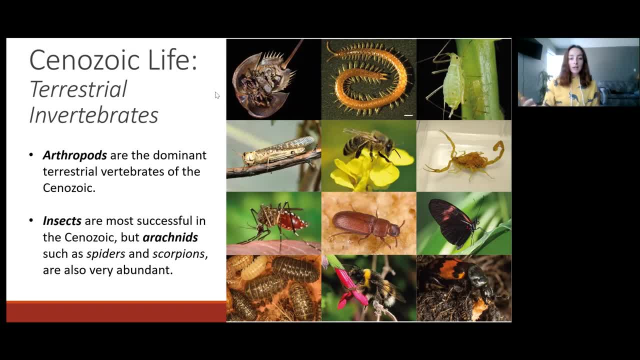 in the Cenozoic And I just realized that this slide says dominant vertebrates. Pretend like that says invertebrates. Arthropods are not vertebrates, So insects are the most successful in the Cenozoic, but arachnids such as spiders and scorpions are also very abundant. So, moving on to marine, 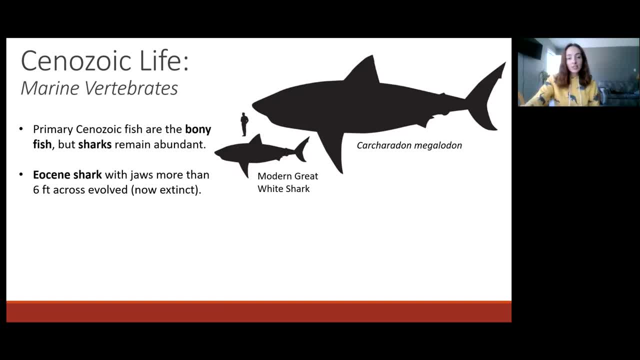 vertebrates. now we have most of the fish in the Cenozoic being bony fish. However, some cartilaginous sharks remained abundant and continue to remain abundant today. There is one difference in today's sharks than in, for example, the Eocene sharks. During the Eocene sharks with jaws more than six. 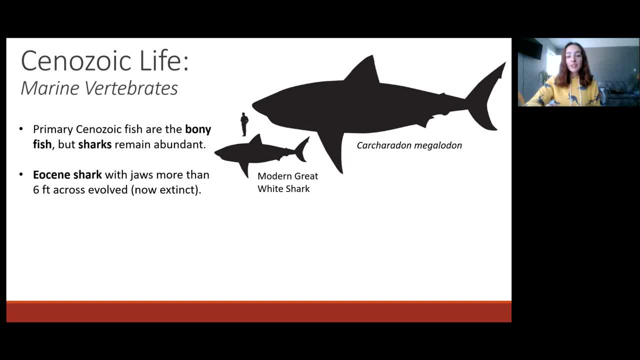 feet across had evolved and these were called cartilaginous megalodon, And I'm sure you all have heard of megalodon fish. Thankfully, they are now extinct. My goodness, that would be terrifying. Now, regarding marine reptiles, we talk in the Mesozoic about marine reptiles that 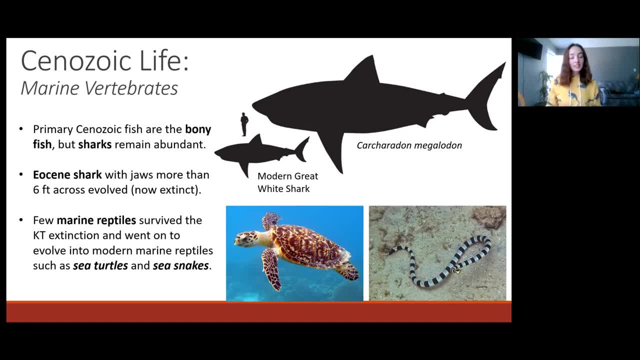 are today's marine mammals. However, after the KT extinction, only a few marine reptiles had survived, and these went on to become things that we know in the modern day to be sea turtles and sea snakes, And therefore the niche that had been filled by Mesozoic marine reptiles could now be. 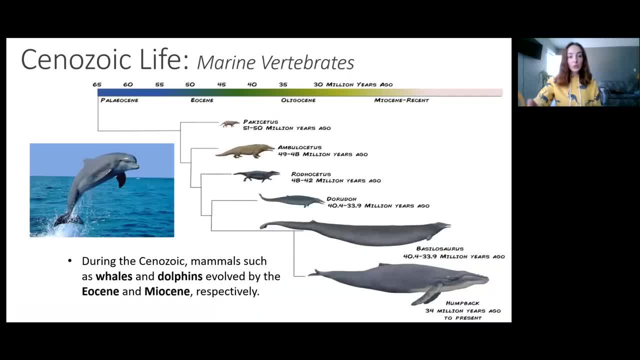 filled by marine mammals. So that brings us to the next slide of marine invertebrates, which is cetacean evolution. Cetaceans are just marine mammals, like whales, dolphins and other porpoises, And during the Eocene they were also called marine reptiles, So they were called marine. 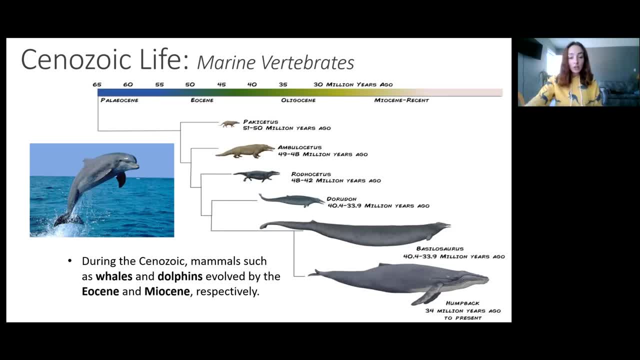 reptiles And during the Eocene, whales evolved And during the Miocene dolphins evolved. And it's just kind of crazy to think that mammals had evolved from fish that had learned to walk on land and become tetrapods And then, millions of years later, mammals that had become primed to. 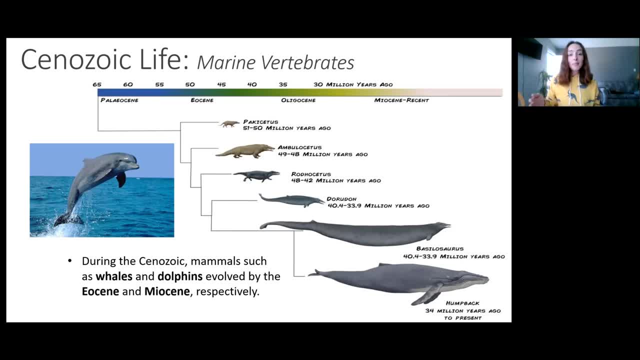 walk on land, decided to go back into the ocean and become marine mammals, And this diagram shows the example of whales which started from animals such as Pakicetus, which is this first picture, and tetrapod that looked somewhat like this evolved into each one of these stages of whale. 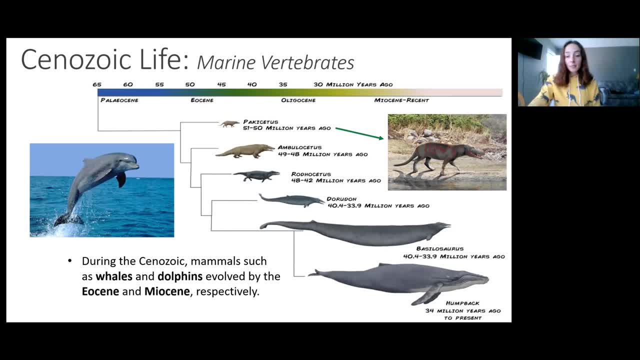 evolution before becoming what we know today as humpback whales, And there's obviously a lot more intermediate stages in between each one of these major stages. But it's just crazy how much we have in the way of whale preservation and all the stages that point to this, which seems like the 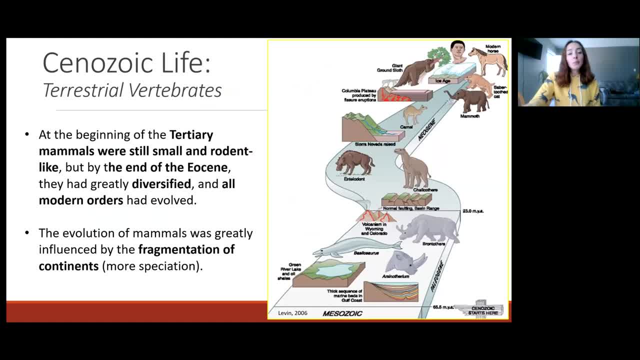 most unlikely pathway, but it is, And it's so cool. So, moving on to terrestrial vertebrates, like we said earlier, mammals were dominant And that's why the Cenozoic is sometimes referred to as the age of mammals. 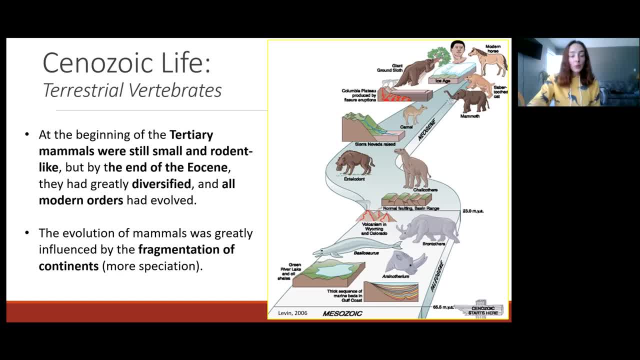 However, mammals were still small and rodent-like by the end of the Mesozoic, in the beginning of the Cenozoic. However, by the end of the Eocene, they had greatly diversified, And this is largely because of the fragmentation of continents, causing more geographical isolation and therefore more 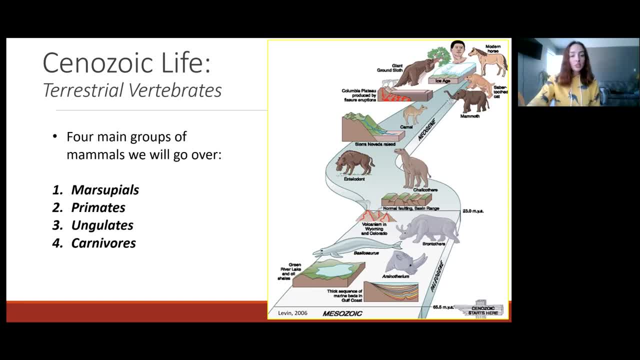 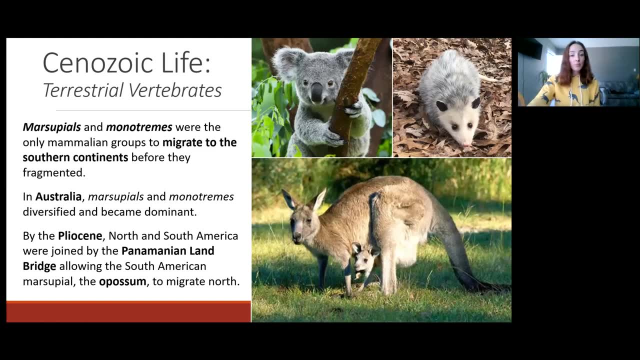 speciation. So the four main mammal groups we will go over in this lecture include marsupials, primates, ungulates and carnivores. First, marsupials and monotremes, which are just mammals. They give birth to really underdeveloped young and then raise it in a pouch. These were the only 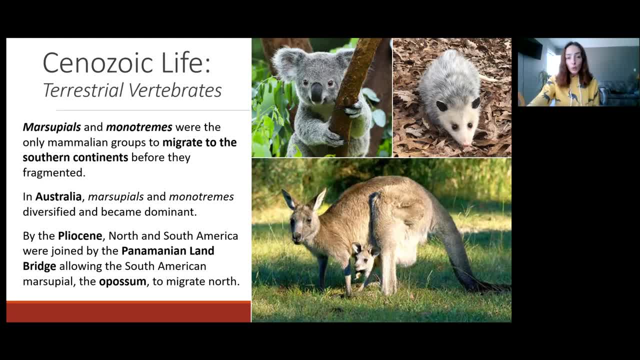 two mammalian groups to migrate to the southern continents before they fragmented, And this meant that in Australia, marsupials and monotremes diversified and became dominant and still remained dominant, And by the Pliocene North and South America had been joined by the Panamanian. 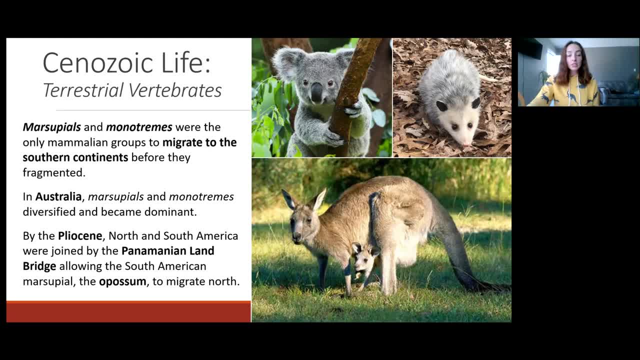 land bridge allowing South American marsupials such as possums to migrate north, And now possums are the most successful marsupial in North America. Moving on to primates, primates had evolved by the latest Cretaceous in the late Mesozoic And by 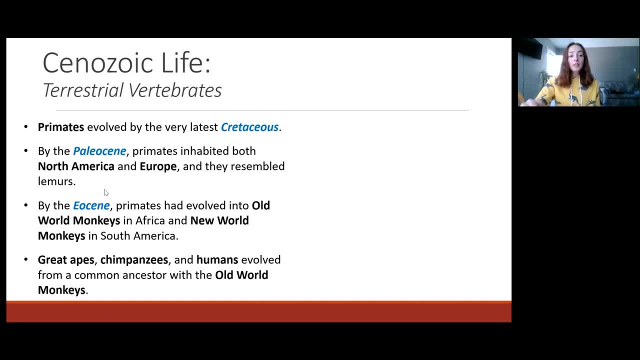 the Palaeocene, in the early Cenozoic primates had inhabited both North America and Europe, and they resembled lemurs. However, by the Eocene, primates had evolved into Old World monkeys in Africa and New World monkeys in South America, which are just the terms we use to describe these two. 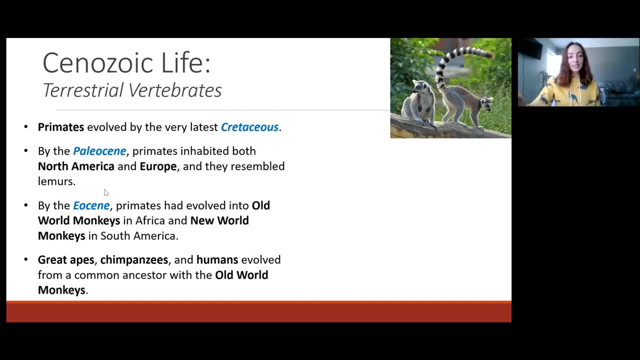 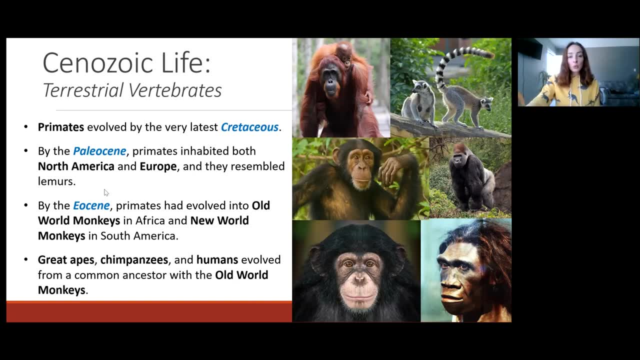 physiologically different groups of primates. The old and new has nothing to do with time, But regarding great apes, chimpanzees and heo- humans, we all evolved from a common ancestor, with old world monkeys Moving on to ungulates. 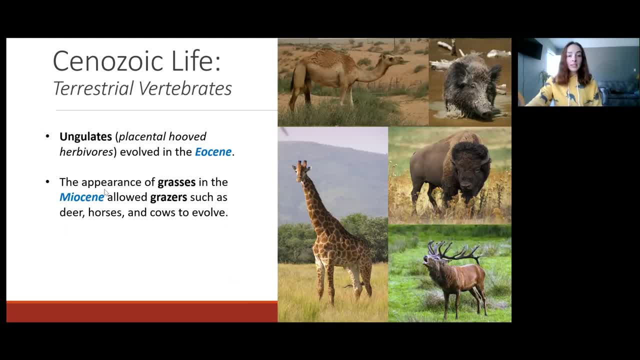 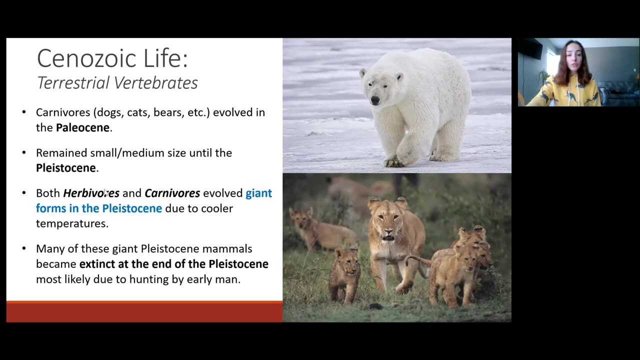 ungulates are just placental hooved herbivores. These evolved by the Eocene, and the appearance of grasses in the Miocene allowed grazers such as deer horses and cows to evolve. Regarding carnivores such as dogs, cats, bears, etc. these evolved by the Paleocene, so very early in the 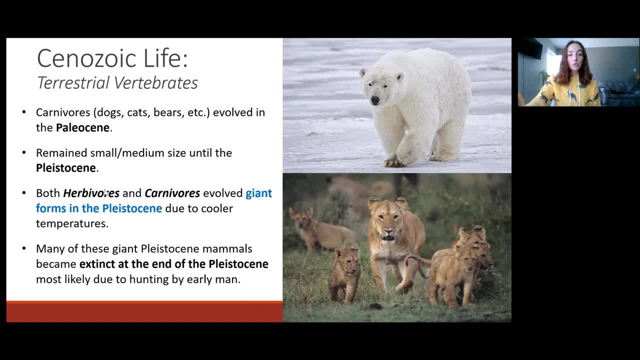 Cenozoic and remained small to medium size until the Pleistocene. So throughout most of the Cenozoic these were small to medium sized. However, by the Pleistocene a lot of things got mega-sized, including not only some of these carnivores, but also some of the herbivores we were just 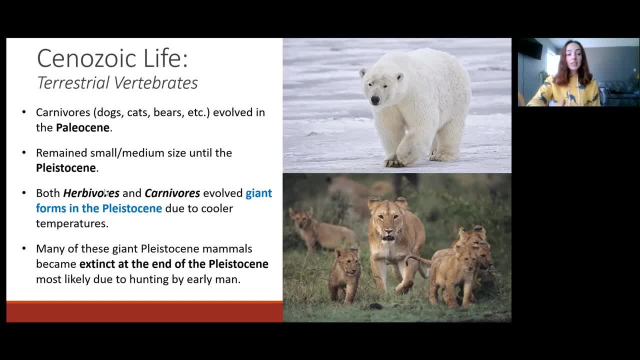 talking about. They evolved into giant forms in the Pleistocene due to cooler temperatures, and this is because large bodies have smaller surface area per volume and can more easily conserve heat, And a couple examples of some of these megafaunas include things like mammoths. 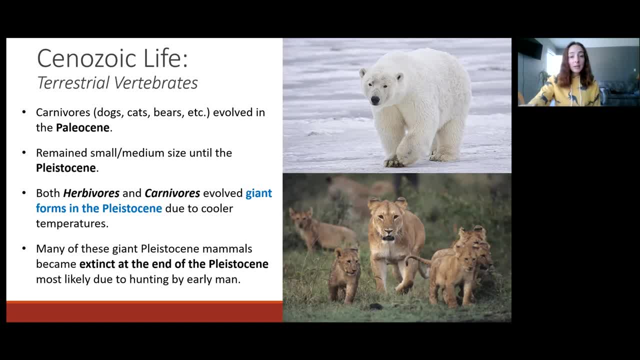 and giant ground sloths, But unfortunately many of these giant Pleistocene mammals became extinct by the end of the Pleistocene And it's debated among researchers whether this is due to hunting by early man or whether this is due to rapid climate change and vegetation change that 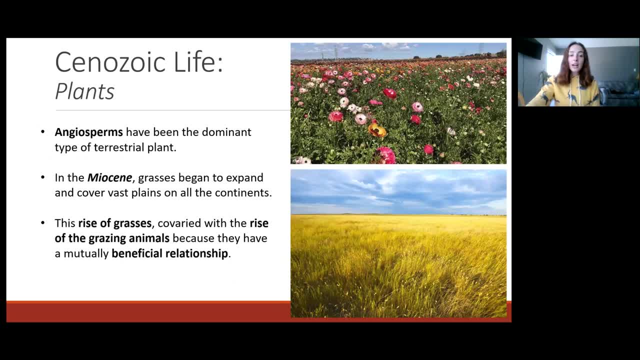 had occurred at the end of the Pleistocene. So, moving on to plants, we have angiosperms, or flowering plants that we talked about last time in the Mesozoic video evolving in the Cretaceous. They then went on in the Cenozoic to become the dominant type of terrestrial plant. 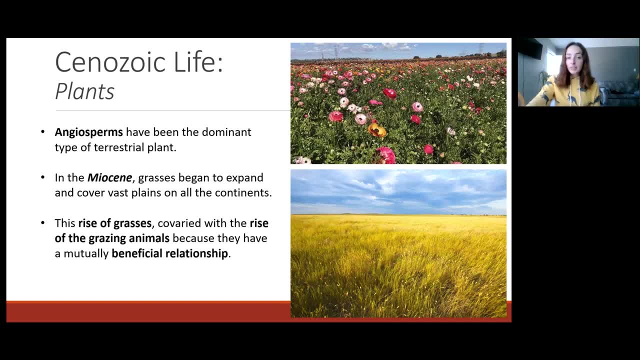 and along with that they did a lot to contribute to the evolution of pollinating insects. And then in the Miocene grasses began to expand and cover vast plains of all continents And the rising grasses, like I mentioned earlier, co-varied with the rising grazing animals.